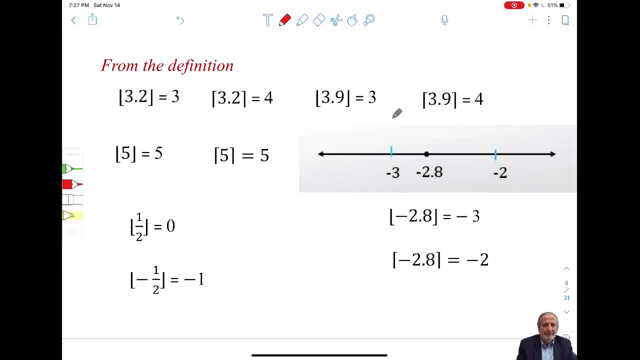 is again 3.. That's rounding down. The ceiling function of 3.9 is 4.. Now, when you have the floor function of an integer, 5 is 5. And the ceiling function of 5 is 5.. The floor function of x is here. 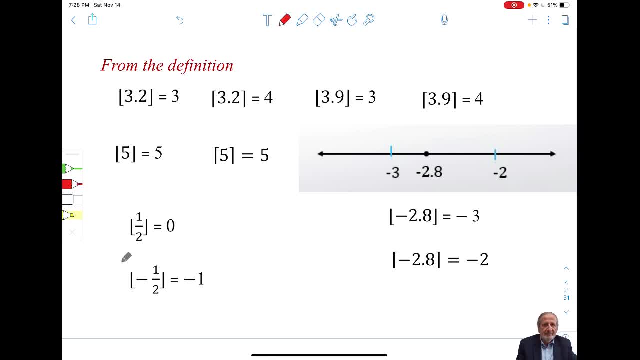 The ceiling function at one half is zero. So if you put your zero is here, one here, And this is your x is one half and the floor function of one half is zero. The ceiling function of one half is one Here is minus 1 half. so you have zero minus 1.. 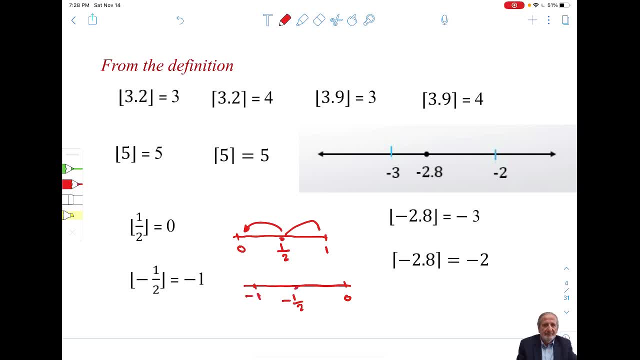 And that's your minus one half. Now the floor function of minus one half is minus one. The seating function of minus one half is zero. Look here at minus 2.5 is between minus 3 and minus 2.. So minus 3 is the floor function and minus 2 is the seating function. 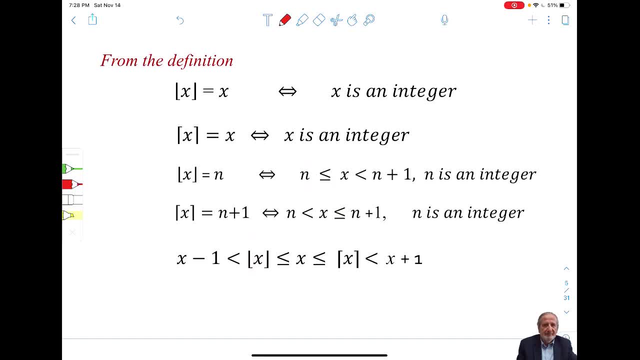 Now here are some important properties. They're really clear from the definition. X is a, X is an integer, Then the floor function of X is X and the seating function of X is X And vice versa. And if N is between greater or equal than, if X greater or equal than N and less than N plus one half, then the floor function of X is X. 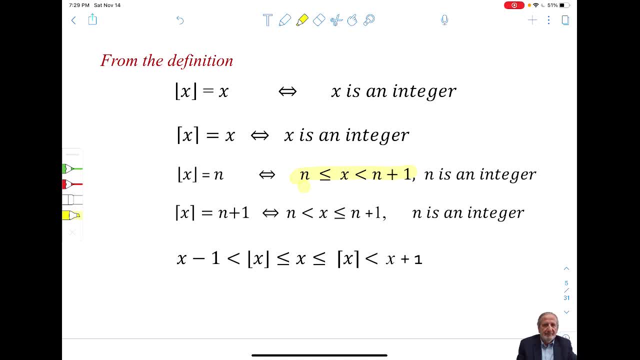 So if N is between greater or equal than N plus one, N is an integer, then the floor function of X is N. The floor function of X is N, and vice versa. And now, if X is greater than N and less or equal than N plus one, then the seating function of X is N plus one. 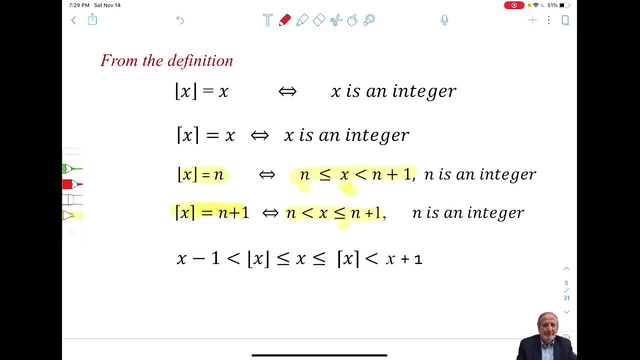 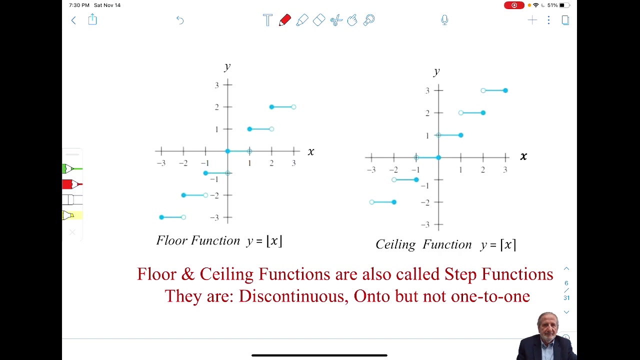 And this is. you can easily see that this one here, X is less or equal than seating. function of X less than X plus one, And X is greater or equal than floor. function of X greater than X minus one. Now, these functions are called also step functions because they look like steps And they are discontinuous onto, but not one to one. 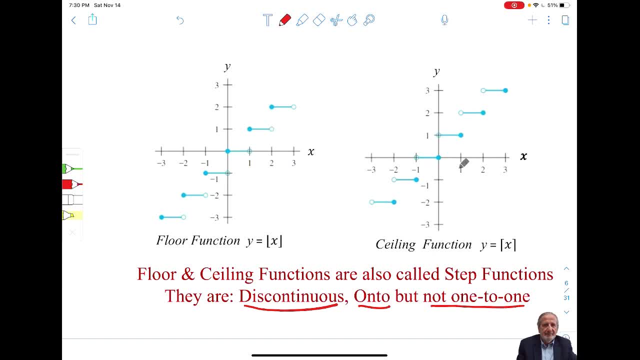 And you notice here, when X starts from zero, the seating function is zero. As soon as you move a little bit here it jumps to one like 1.1, 1.2,, 1.3, the seating function is sorry: zero one, zero two, zero three. the seating function is one. 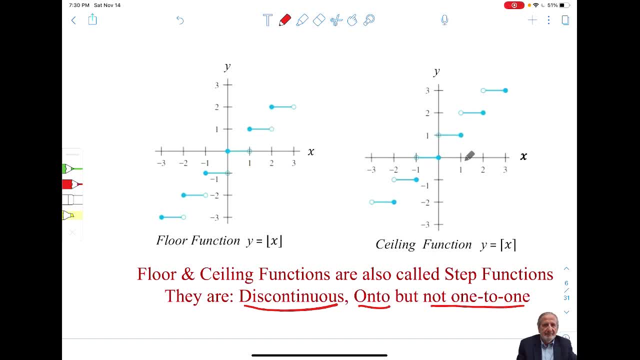 One is one. Now, once you go a little bit beyond one- like 1.1,, 1.2,, 1.3, it jumps to two, And then here it jumps to three, and so on and so forth. Now here's starting to give you some examples now. 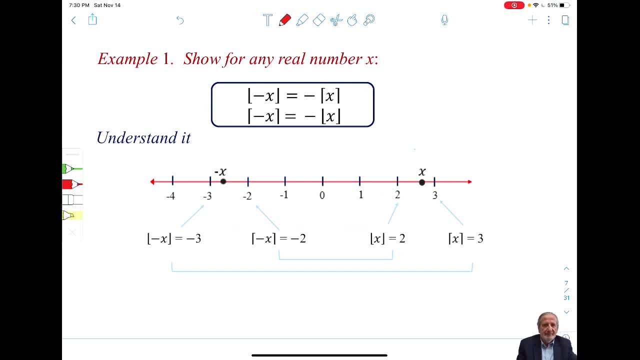 Important examples: The floor function of minus X is minus the seating function of X and the seating function of minus X is minus floor function of X. Sometimes. give yourself some examples to understand what is going on here, What is really being asked. So to understand the question here, I put X here between two and three. 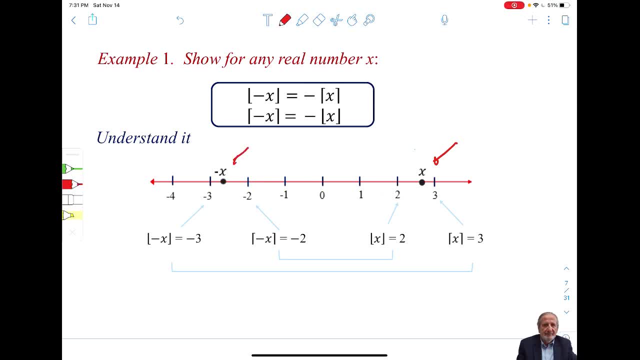 So minus X would be between minus three and minus two. Now X. the seating function of X is three, The floor function of X is two. Look at minus X now. The floor function of minus X is minus three And the seating function of minus X is minus two. 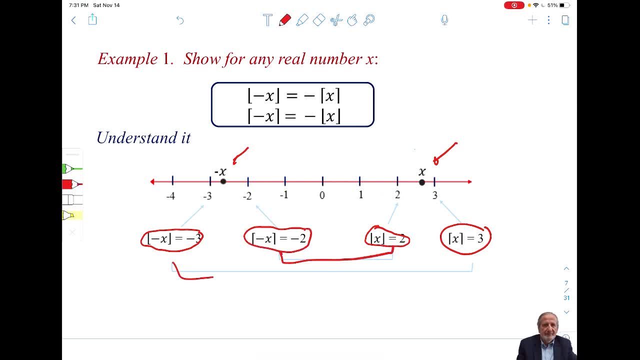 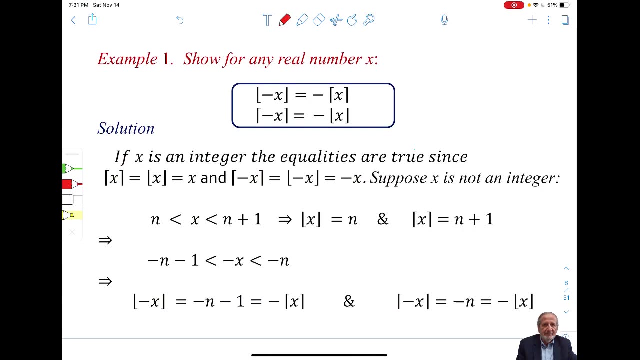 Now compare these two. now Compare these two here, And you see that the floor function of minus X is minus the seating function of X, And the same thing goes for the seating function. Now, how do you prove this? First of all, if X is an integer, then those equalities are true, because, basically, when X is an integer, all these brackets are gone and you see how these are satisfied. 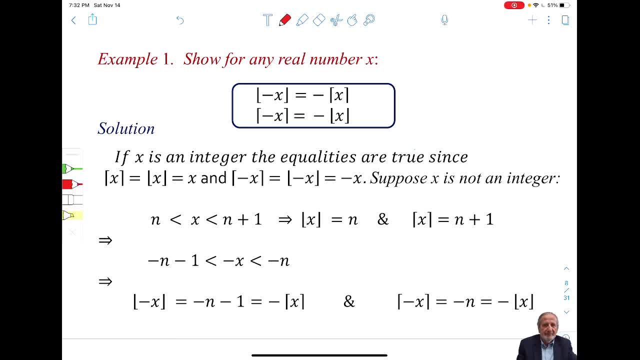 Now we are going to assume now, or suppose, X is not an integer. So when X is not an integer, I'm going to put X between n and n plus one. Okay, So I'm going to put X between n and n plus one. 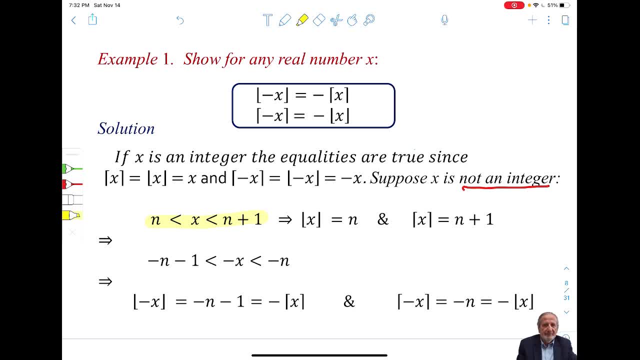 I'm just going to compute now all the terms I need. I need the floor function of X is n. The seating function of X is n plus one. Now take minus X. Minus X is between minus n, minus one and minus n. 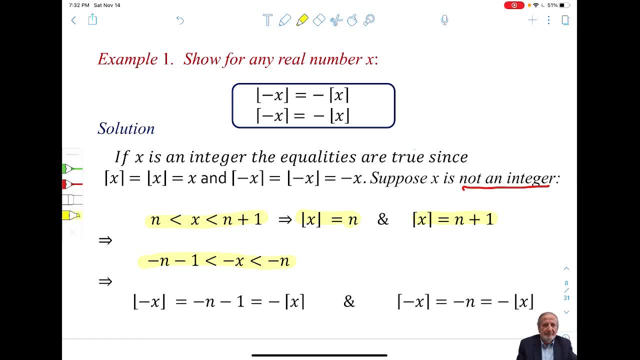 So now, what is the floor function of minus X, minus n, minus one, Which is Minus the seating function of X? And now the seating function of minus X is minus n, And minus n is minus the seating function of X, Minus the seating function of X. 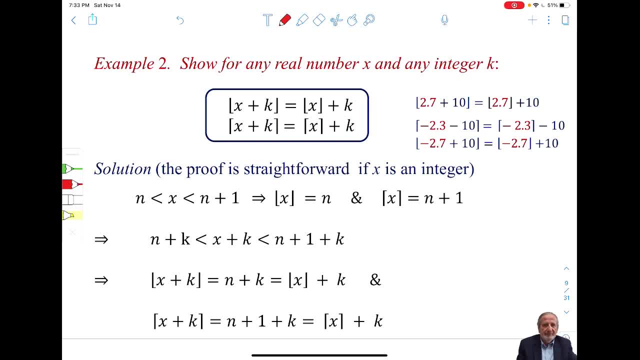 Now, this is a very important property That we are going to be using. We are going to be using quite a bit in this lecture. If you have any X, any real number X and any integer K- X plus K- the floor function is the floor function of X plus K. 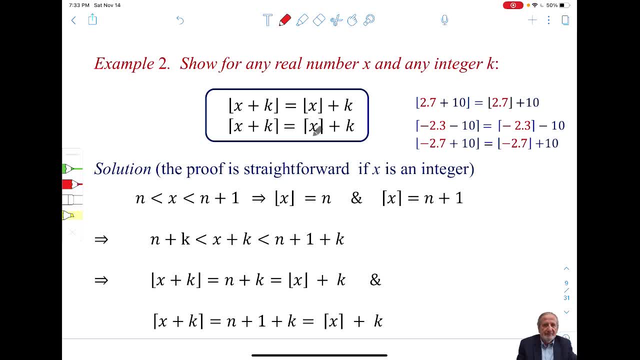 And the seating function of X plus K is the seating function of X plus K. It's as if you're taking this and getting it outside of the bracket. You're taking this and getting it outside And you're taking this and getting it outside of the bracket. 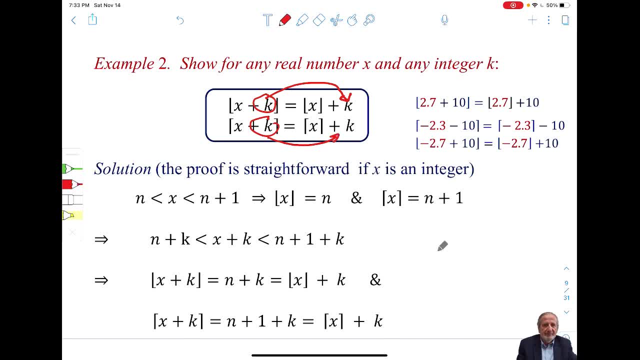 To understand that you can see in this example: square root of the floor function of 2.7 plus 10 is the floor function of 2.7.. And you add 10 to it, So the floor function of 2.7 is 2 plus 10.. 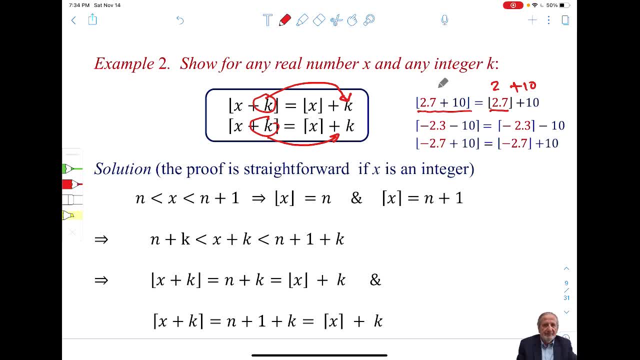 Here. here you have 12.7,. the floor function of 12.7 is 12, and they're equal. The same thing for the other, for these other examples. Now, how do we prove this? properties is very simple. 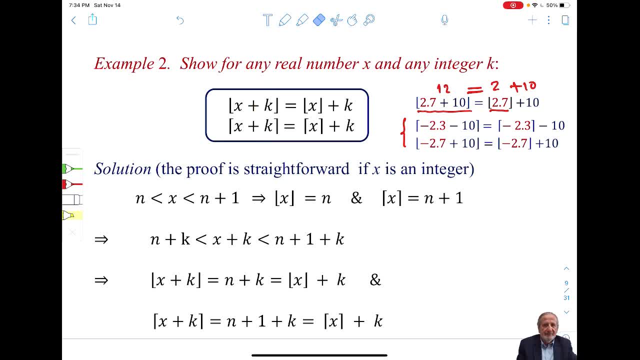 Now if X is integer, then those are equal, Because the brackets really are gone And those are equal. So this is straightforward. Now we're going to suppose X is not an integer. So when you say X is not an integer, you put it between N and N plus 1.. 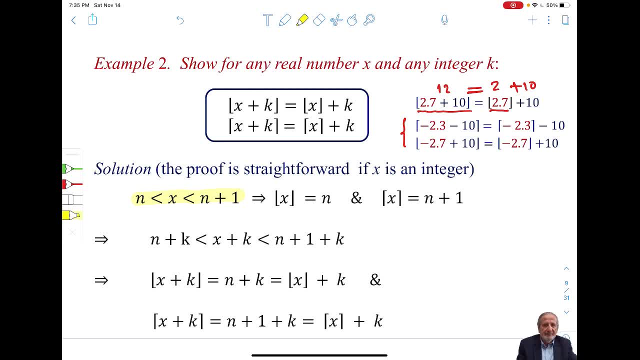 And let's do some calculation. Now, what's the floor function of X is N. What's the seating function of X? is N plus 1?. Now I need X plus K, X plus K, so I add K to both sides. 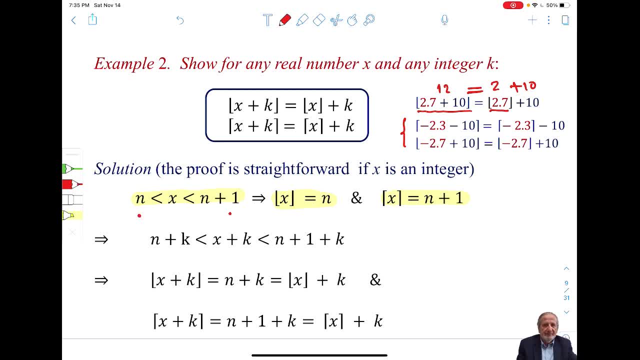 I add K to both sides, this side and this side. So X plus K Will be greater than N plus K, less than N plus 1 plus K. So this one here actually is N plus K plus 1.. So N plus K is between two consecutive integers: N plus K and N plus K plus 1.. 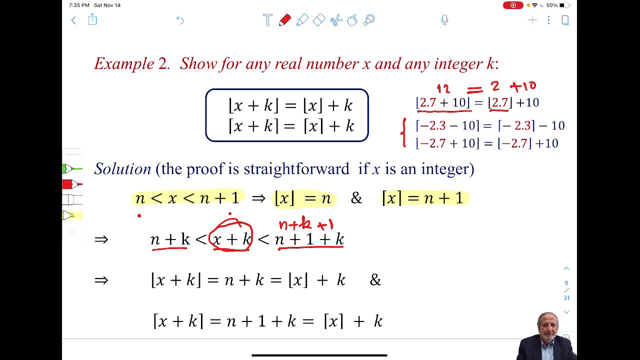 Now I can compute the floor function and the seating functions of N plus K. So the floor function of N plus K is this: Okay, and you notice that N plus K. so what is the floor function of X plus K? That's the left-hand side, okay? 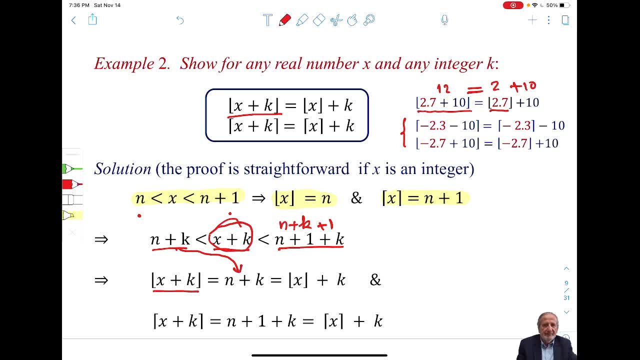 That's the left-hand side. What's the right-hand side? floor function of X plus K? Because floor function of X is N see Plus K. So the left-hand side is equal to the right-hand side. The same thing now. 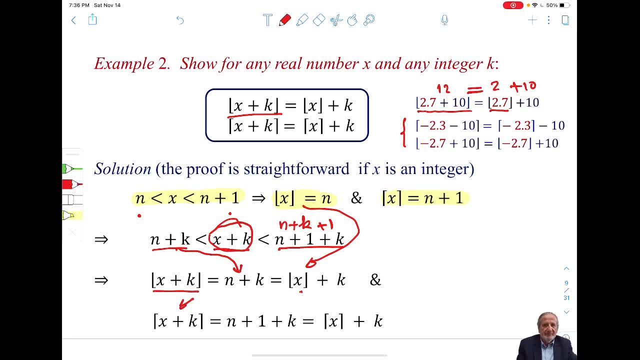 What is the seating function of N plus K? is N plus K plus 1, N plus K plus 1, N plus 1 plus K? see So and N plus 1 happened to be the seating function of X plus K. 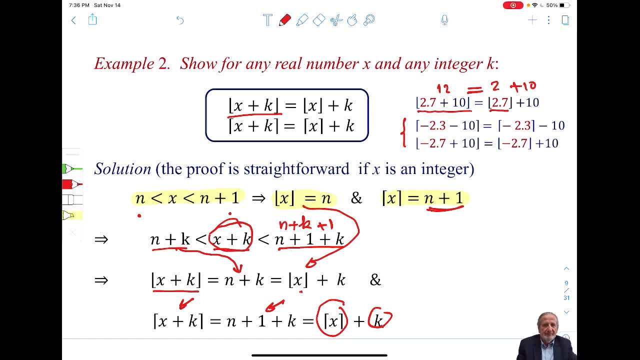 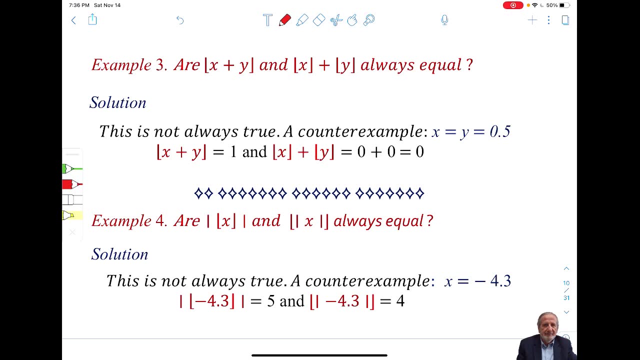 So we proved these two properties. They're very important and you will see we are going to use them quite a bit in this lecture. Okay, So here's a question: Is the floor function of X plus Y and the floor function of X plus the floor function of Y? are they always equal? 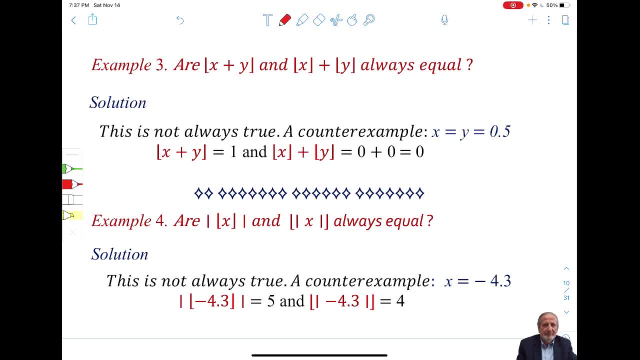 Now you can find the examples where they are equal, but they're not always equal. The answer is no, And then what we do is we find a counterexample. Here I'm giving this counterexample, but I want you to find your own. 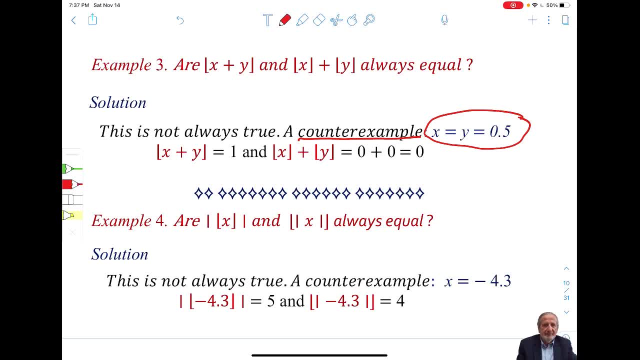 For example, there's a whole bunch of them. So if X plus Y is equal to Y to equal to 0, then X plus Y will be 1.. The floor function will be 1.. The floor function of X is 0.. 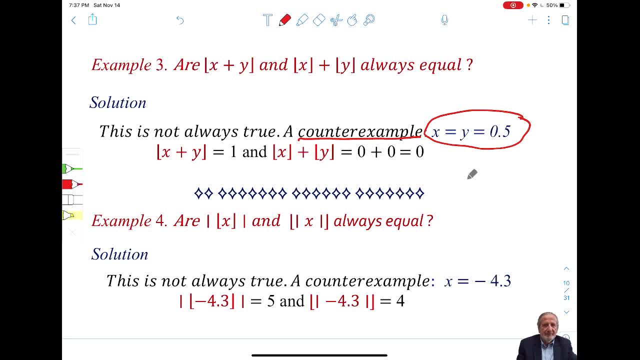 The floor function of Y is 0.. You add them, you get 0.. You get 0. And this 0, and this is 1.. They are not equal. Another question Is the absolute value of the floor function of X. is it the same as the floor function of the absolute value of X? 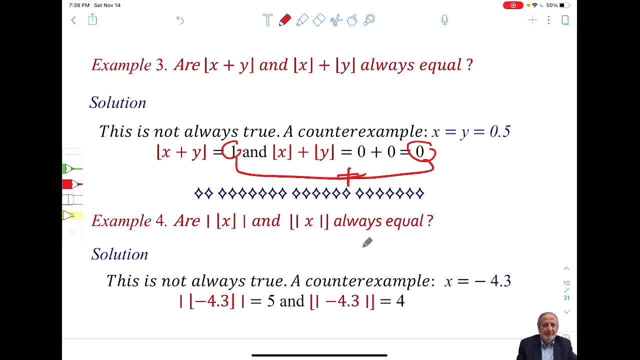 Again, the answer is no And you can give a counterexample Here. I gave you here: X equals to minus 4.3. So when you take the minus 4.3 here and take the floor, function of it is minus 5.. 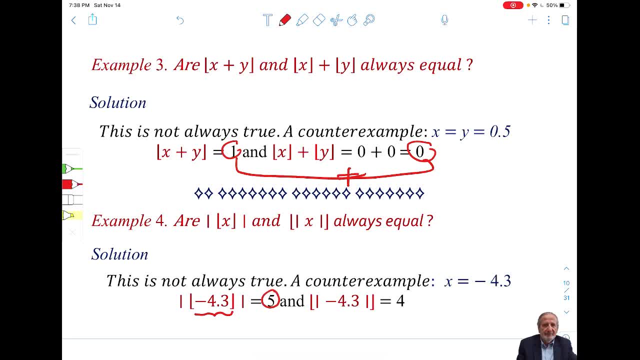 You take its absolute value, It will be 5.. But if you take the absolute value of minus 4.3, it will be 4.. And the floor function of 4 is 4.. And you see 4, 5.. 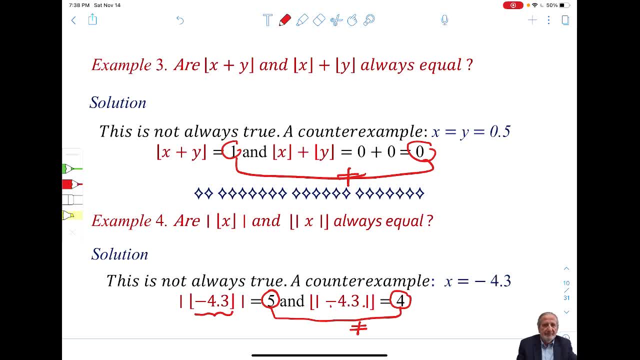 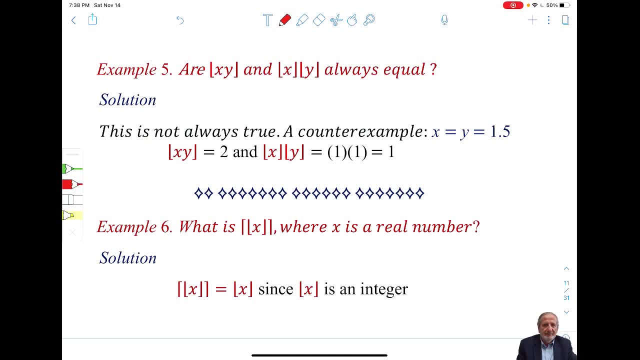 They are not the same. Another question: The floor function of XY and the floor function of X times the floor function of Y. are they always equal? Again, the answer is no. Here is an example. Here I take: X equals, Y equals 1.5.. 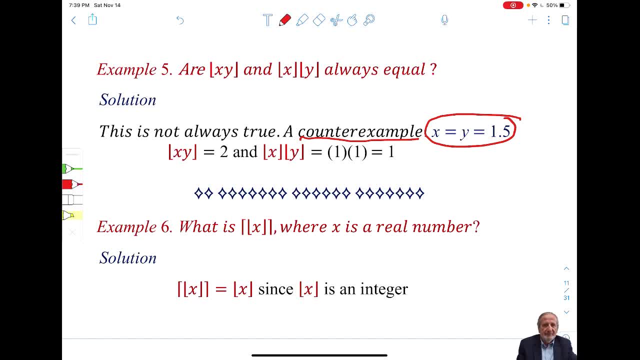 So when you multiply X by Y, X times Y, you get 2.25.. And the floor function will be 2.. But if you had what is? the floor function of X is 1, the floor function of Y is 1.. 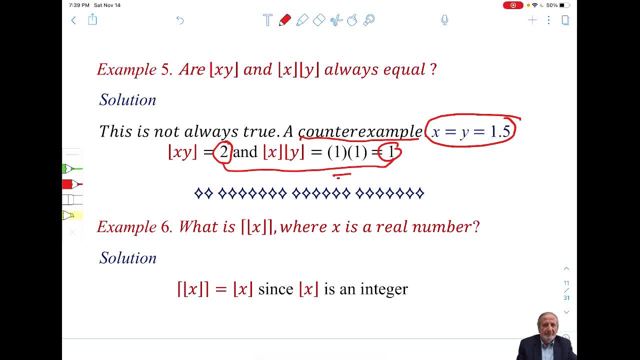 1 times 1 is 1.. Again, see, 2 is not the same as 1.. They are not equal. Now, what is The ceiling function of the floor function of X for any real number? X, Now, remember, this is an integer. 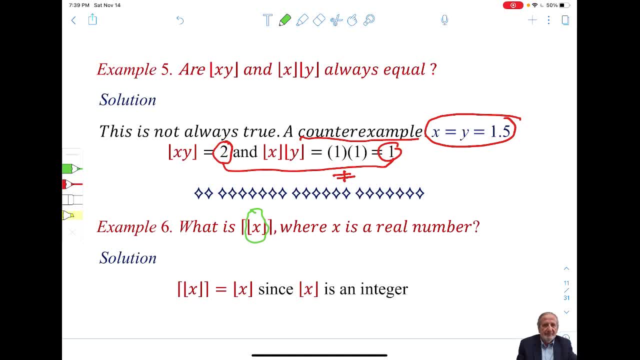 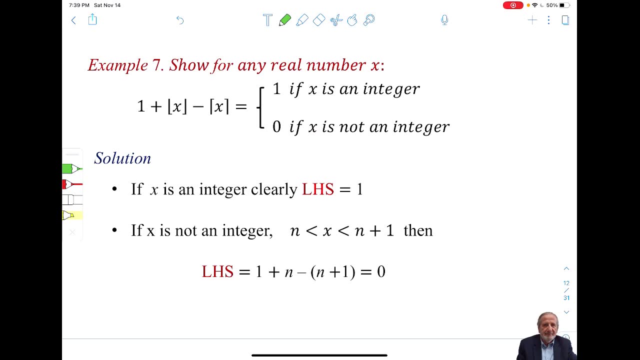 So the ceiling function of an integer is itself. So you get this as an answer. Now here is another example. Here is another example. So for any real number, X, 1 plus floor function of X, minus ceiling function of X is 1 if X is an integer and 0 if X is not an integer. 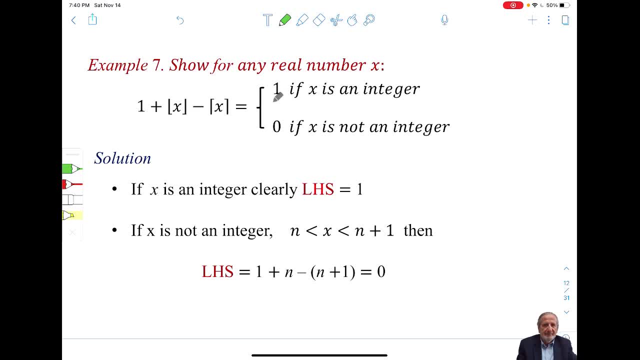 So this here is 1 when X is an integer and 0 when X is not an integer. Well, it's very simple, because if X is an integer, the brackets are gone here and X minus X is 0. So you get 1.. 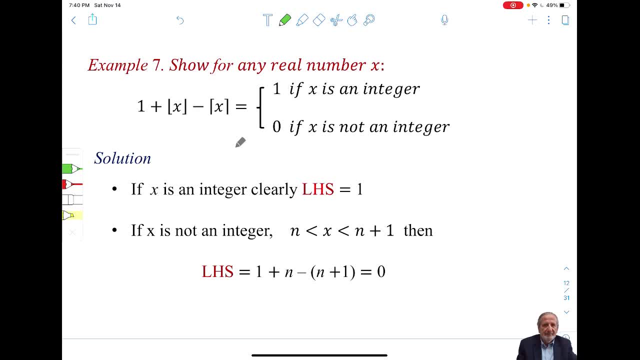 Now the question is Now is when X is not an integer. So again, X is not an integer. See, I put X between N and N plus 1.. So now, what is the left-hand side? The left-hand side. 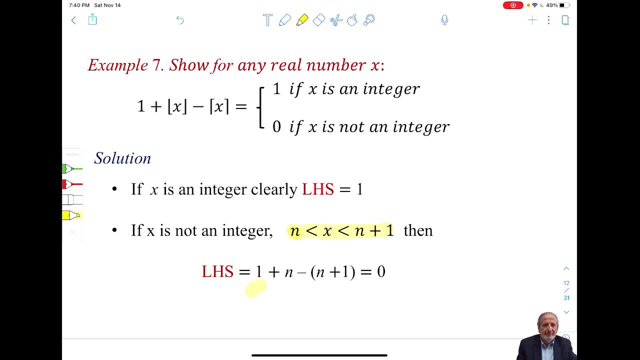 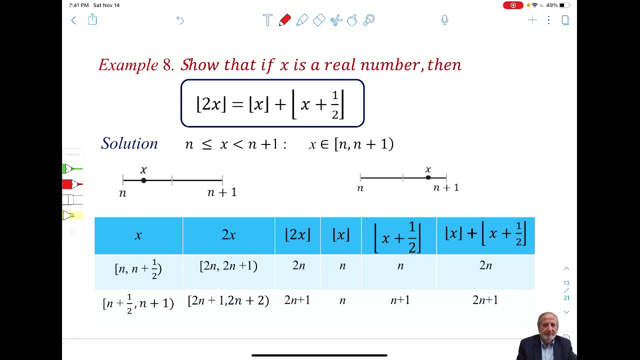 What is 1?? Is 1 plus floor function of X, N minus ceiling function of X? and you see, the answer is 0.. Now here is another example. We need to show that if X is a real number, then floor function of 2X is equal to floor function of X plus floor function of X plus 1 half. 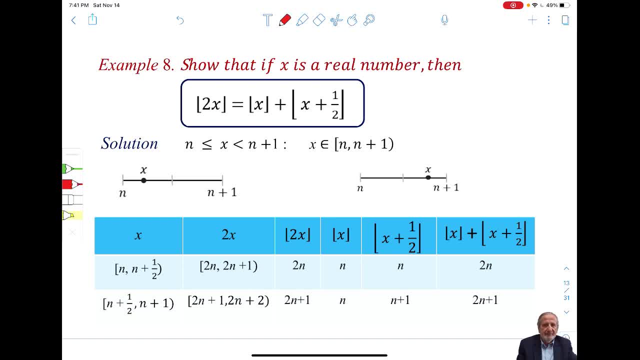 Now I just want to remind you About some notation. When we say X between N and N, plus greater or equal than N and less than N plus 1, it's the same as saying X belongs to this interval Closed. Closed on this side and open on this side. 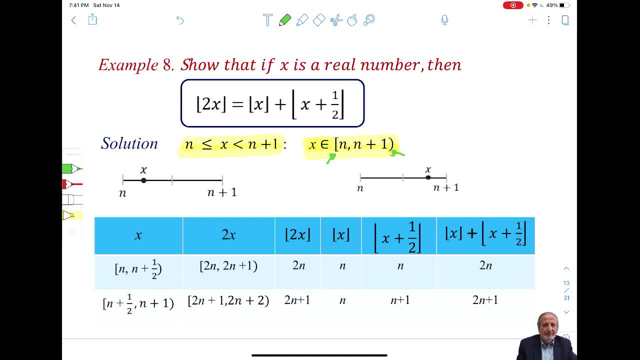 Okay, That means between 2, between N and N plus 1, N is included, N plus 1 is not included. Now the problem here is You have, Because of this, 1 half. what happened if X is in this area here? 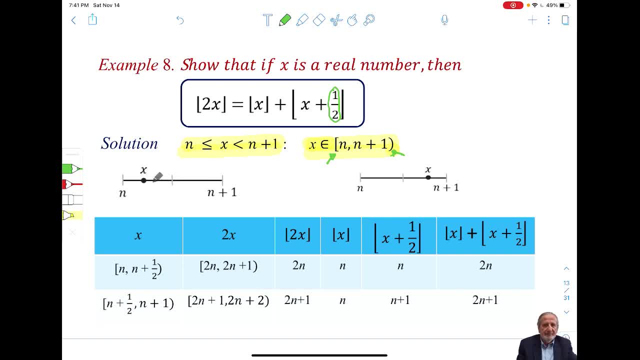 If X in this area here, when you add half to it, you will still in this interval and the floor function will be N. But when X is in this area here and you're adding half to it, it jumps to here and then the floor function will be N plus 1.. 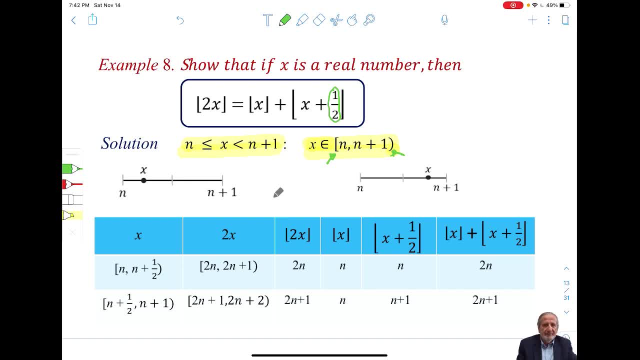 That's why we are going to distinguish two cases, Case 1.. Case 1 is here: X between N and N plus 1 half, And the other case X between N plus 1, N plus 1 half and N plus 1.. 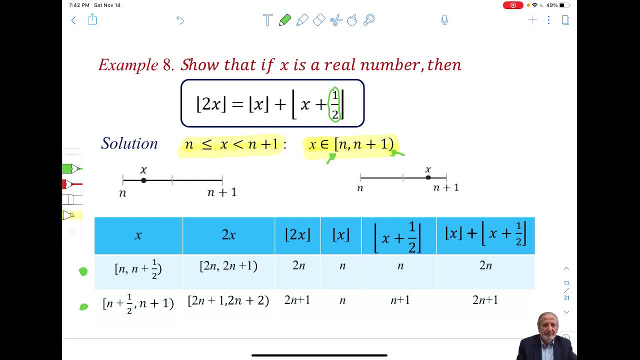 Now, this way, I cover all the values of X between N and N plus 1.. So this is X. Now you find 2X. You multiply this by 2. You get this Very simple. Now I have this and I have this. 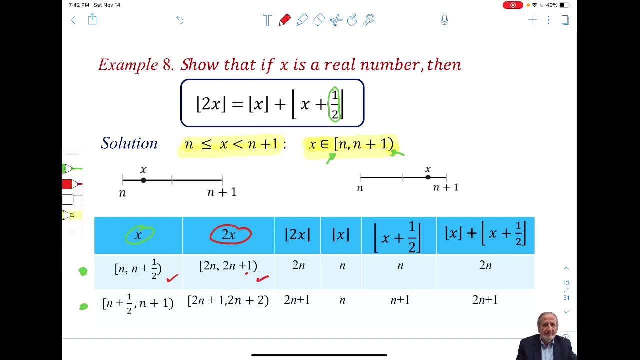 I can now compute. the floor function of 2X is 2N. Floor function of X is N. Now I'm adding to X 1 half. I'm adding to X 1 half. So I am now here When I add 1 half. I am in this situation. 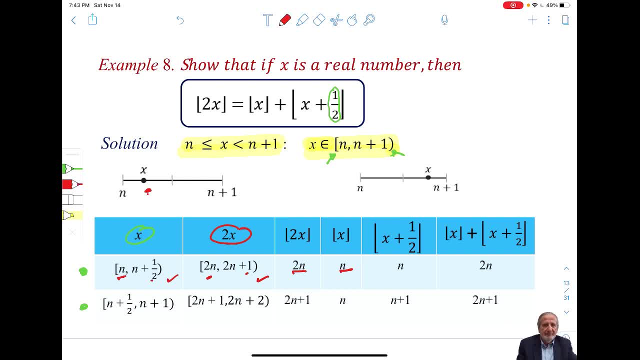 I am here now When I add 1 half, I'm going to still be here and the floor function will be N. Now you add these two, You get 2N. You get 2N here and they're equal. 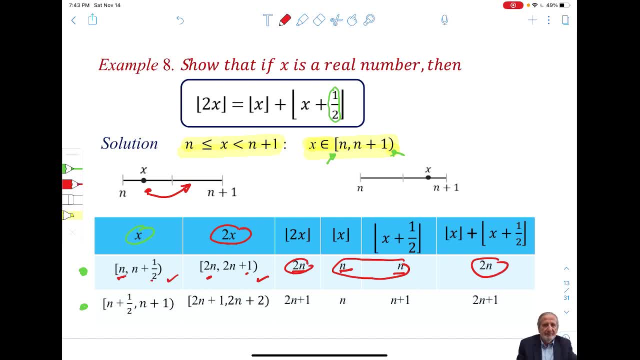 Now we move to the second possibility. X is in this area here. Okay, So again you find 2X. It will be this here. Now, what is the floor function of 2X? Floor function of 2X is 2N plus 1.. 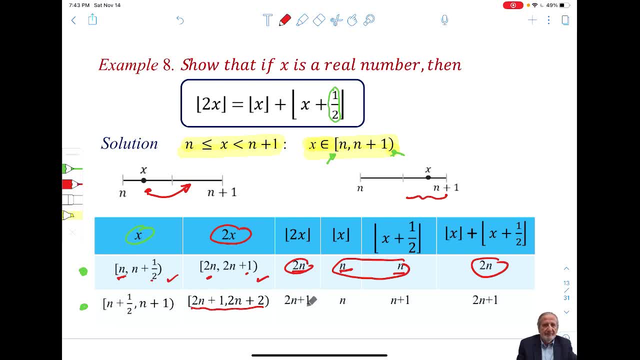 You can see that right here: 2N plus 1.. That's the floor function. Now what is the floor function of X? X is here. Floor function of X is N, Now X plus 1, half. Here's the problem now. 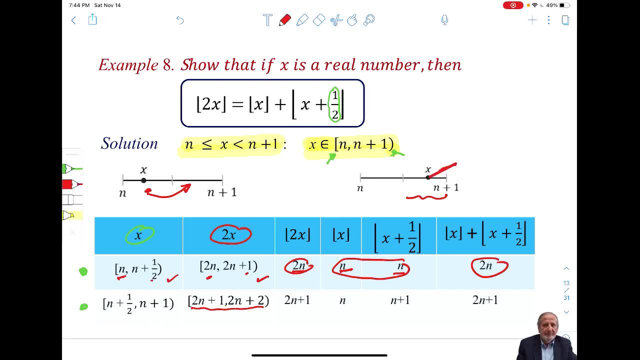 When you add 1 half to this, it's going to, It's going to go out that way, And then when you take the floor function, it will be N plus 1.. And plus N, 2N plus 1,, 2N plus 1, they're equal. 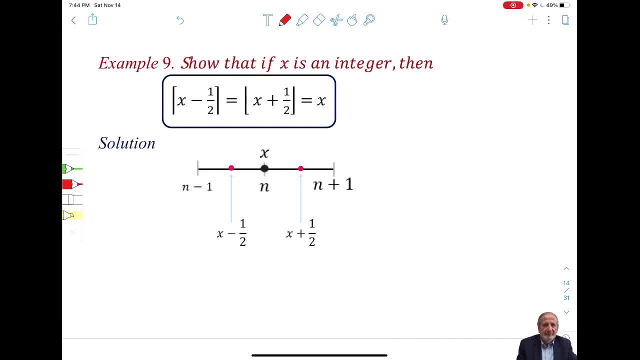 Now here's another example. now Show that if X is an integer, then seeding function of X minus 1 half Is equal to the floor function of X plus 1 half is equal to X. So this is really simple, because here's X is right here as an integer. 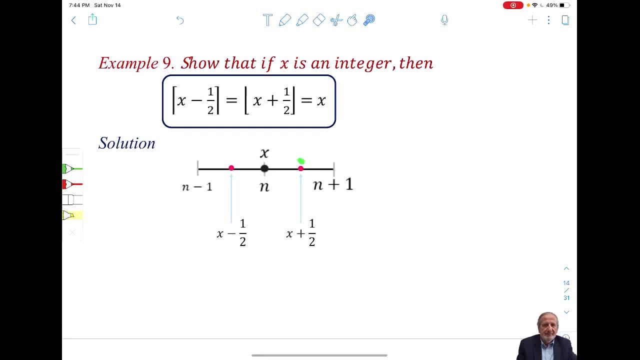 So X plus 1 half takes you to here. X minus 1 half is here Now. if you take this X minus 1 half and take the seeding function of it, it takes you back to N. If you take here X plus 1 half, this one here, and take that floor function of this, it takes you back to N. 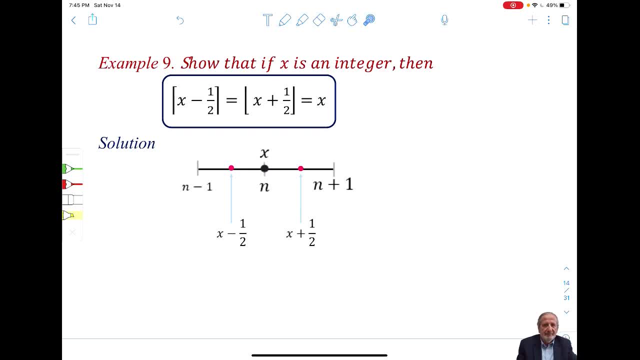 It's very simple Now: if X is in the middle is N plus 0.5, N is an integer, then these are not equal. See, this is not equal. So again now, X is right in the middle here. 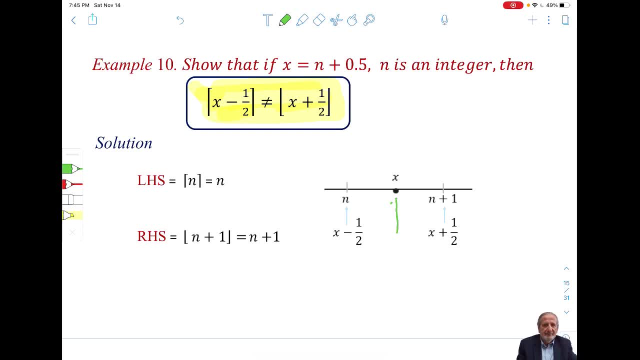 See what I did. X is right here in the middle. When you add 1 half to it, you get to this point, And when you subtract 1 half from X, you get to this point. here And obviously now the seeding function of this is N. 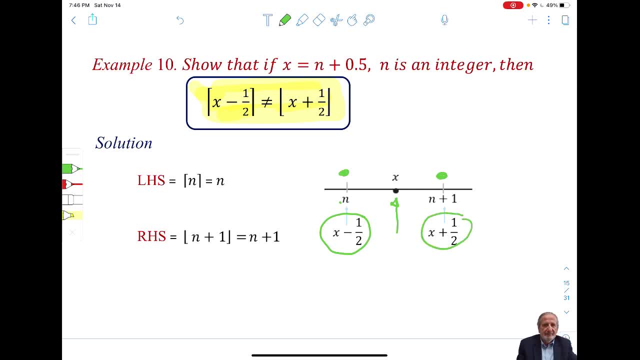 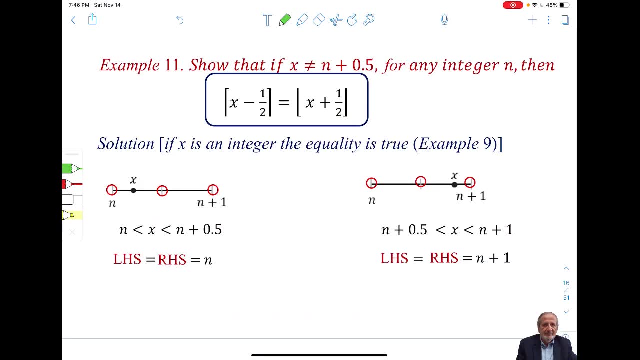 And that floor function of this is N plus 1. So they are not equal. Now, example 11 shows that if X is not equal to N plus 0.5 for any integer N, then this will be true. Then this will be true. 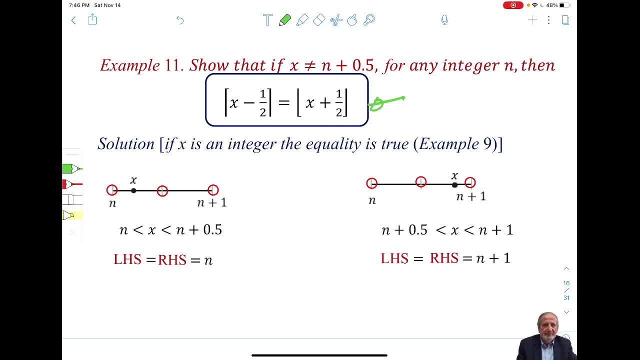 So now the situation is here. I have two possibilities: I have this or I have this. So in this case, here I put: here is X, This is not included. This is not included. This is not included. Okay. 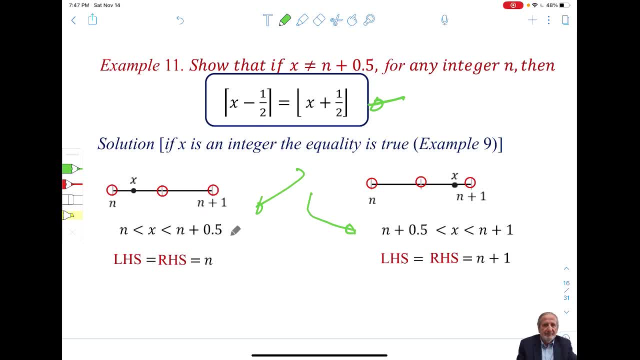 So X is between N and N plus 0.5.. And you can see now what is the left-hand side, This one here: X minus 1 half seeding function. When you take X minus 1 half it takes you to here: 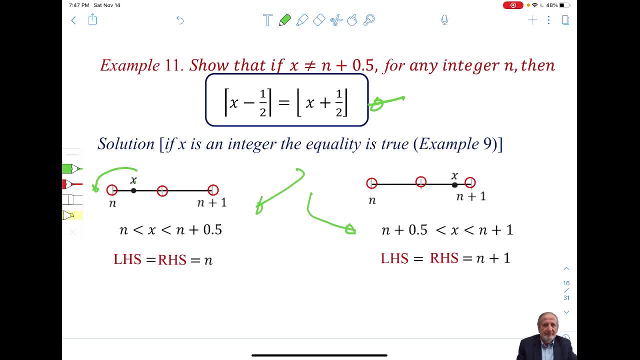 Seeding function is N. Look at the right-hand side: X plus 1 half. X plus 1 half takes you to here. The floor function will be N, So in both cases is N, And you can do the same thing for. 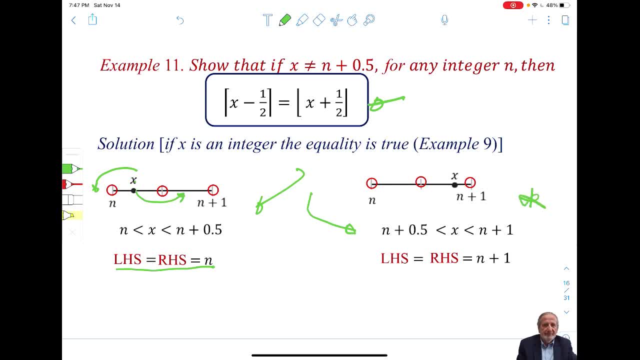 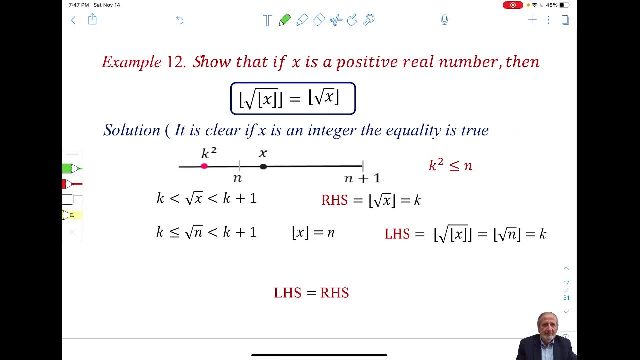 This situation Very straightforward. Now show that if X is a positive real number, then the floor function of the absolute value of the floor function of X is the floor function of the square root of X. Now again, if X is an integer, this is true. 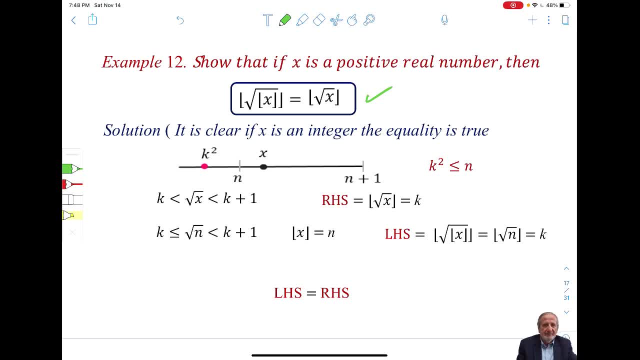 This is straightforward. This is true Now if X is not an integer, so X is between N and N plus 1.. So I put X here between N and N plus 1.. Now I'm going to consider K square less or equal than N. 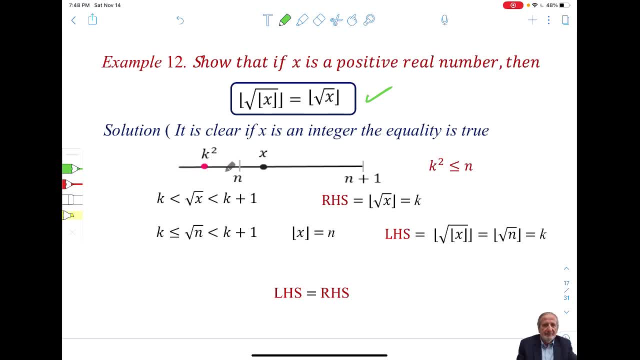 The largest perfect square less or equal than N. Okay Now, in this case, square root of X will be between K and N, K and K plus 1.. Also, the square root of N will be between K and K plus 1.. 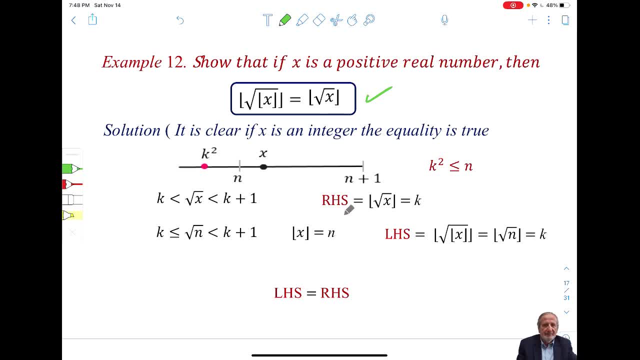 Now all what you have to do is find the left-hand side and the right-hand side. Look at the right-hand side, The right-hand side. here is the floor function of square root of X. Okay, Square root of X floor function is K. 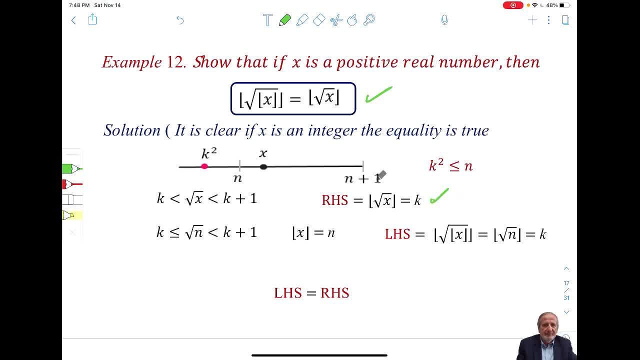 So that's, We did that. Now we need the left-hand side. We need this here. So the floor function of X is N. Floor function of X is N. Now the left-hand side is the floor function of square root of floor function of X is the floor function of square root of N. 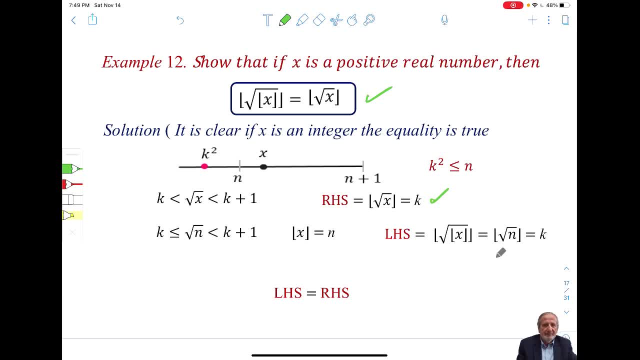 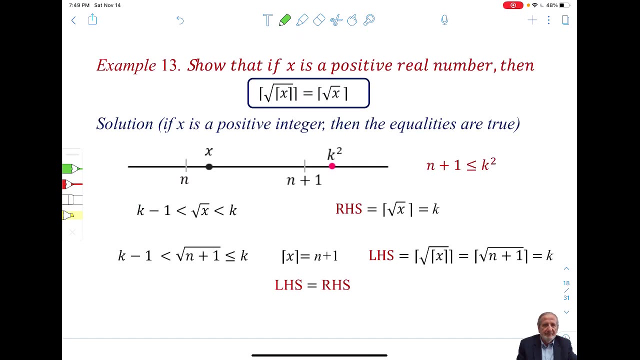 Because the floor function of X is N, And what is this floor function of square root of N? It's K, And in both cases they are equal. Now, this is similar. I will leave it for you to do, But I recommend that you do it first and then you come and look at the answer if you have some problems. 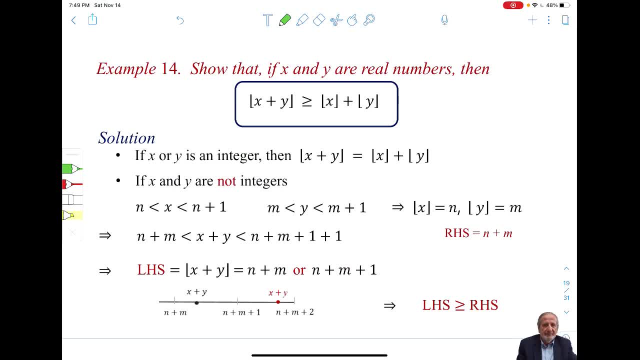 Here's another example: Show that if X and Y are real numbers, then the floor function of X plus Y is greater or equal than floor function of X plus floor function of Y. Now, obviously, if X or Y is an integer, then this will be: 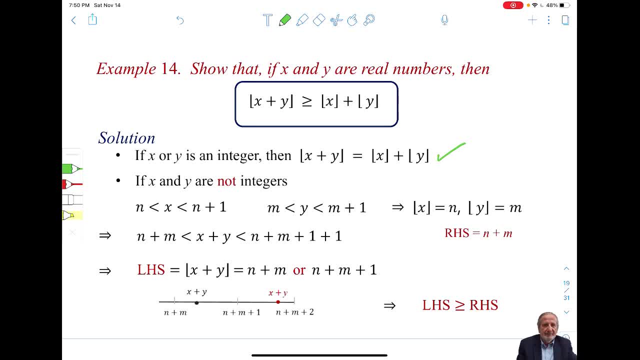 be easy to prove. If X or Y is an integer, then there is no problem. Now, if both X and Y are not integers are not integers. If both of them are not integers, here's what I do. I put one of them here between N and N plus 1.. 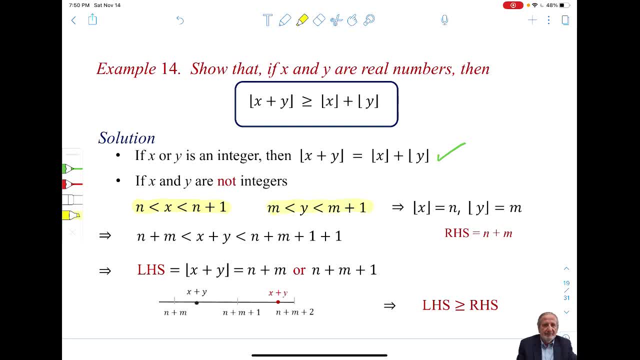 Put the other one between M and N plus 1.. Make sure, Don't use, Don't use this N here and N at the same time. They could be in two different integers. So now from this directly, you can see: 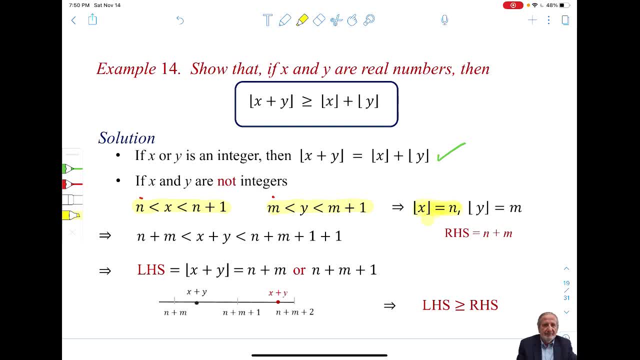 Floor function of X is N, Floor function of Y is M And the right-hand side is N plus M. We got the right-hand side. now We need, We need to. We need to work on the left-hand side. We need to work on the left-hand side. 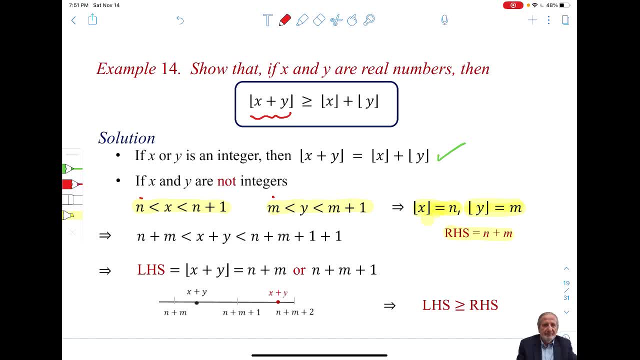 So I add this: X plus Y, And then X plus Y is between N plus 1, M, And between N plus M plus 1 plus 1. Which is N plus M plus 2.. Now I'm saying that in this situation, 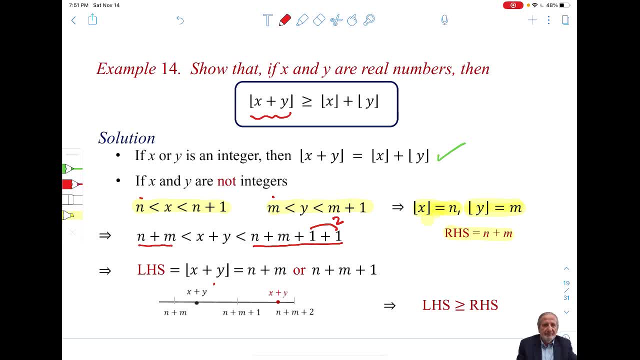 X plus Y. The floor function of X plus Y will be either N plus M or N plus M plus 1.. It depends up where is your X plus Y. Is it in this interval here, Or is it in this interval here? And you see, that means the left-hand side is greater or equal than the right-hand side. 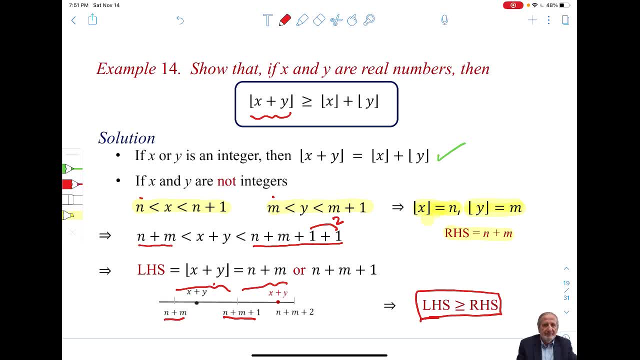 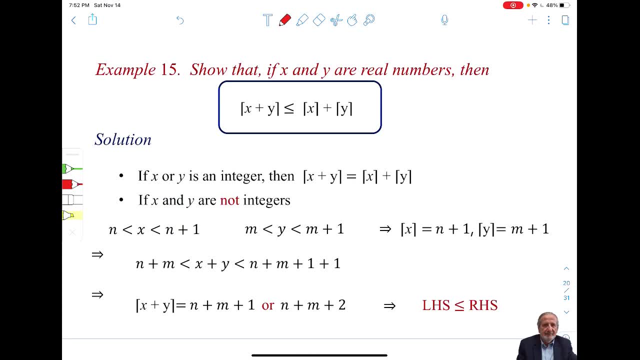 And actually, when it's not equal, it will be greater by only 1.. By only 1.. This is similar. You can do it on your own. The ceiling function of X plus Y is less or equal than the ceiling function of X plus the ceiling function of Y. 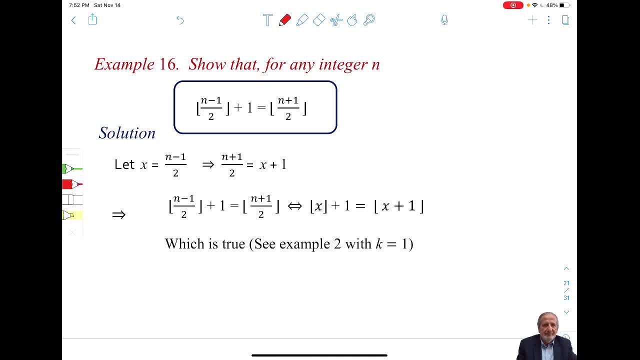 Here's another example: Show that the floor function of N minus 1 over 2 plus 1 is equal to the floor function of N plus 1 over 2.. So what I do here is I take, I took this and called it X. 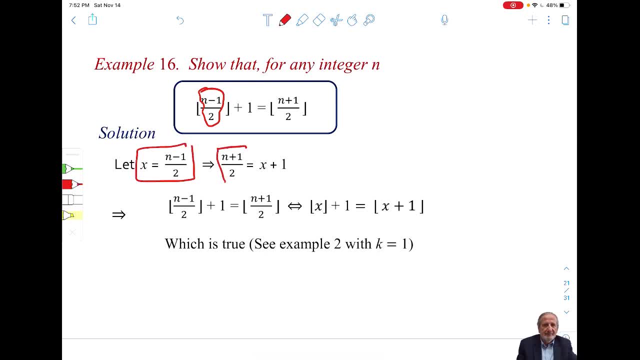 Then when you add 1 to it, The N plus 1 over 1 half is X plus 1.. So now you are asked to prove This, And this is true, because what happened is X. This is This one here. 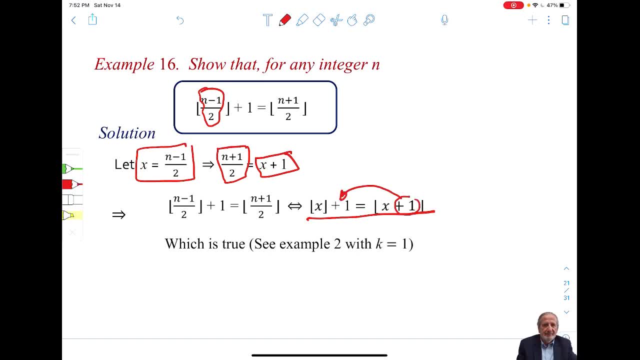 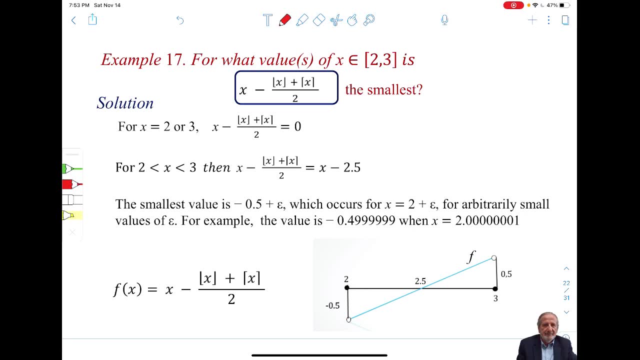 Here is an integer. We take it outside. That's all what we did. Now this is an interesting example for all values of X between 2 and 3.. For what values this quantity is the smallest? Now you notice that when X is 2.. 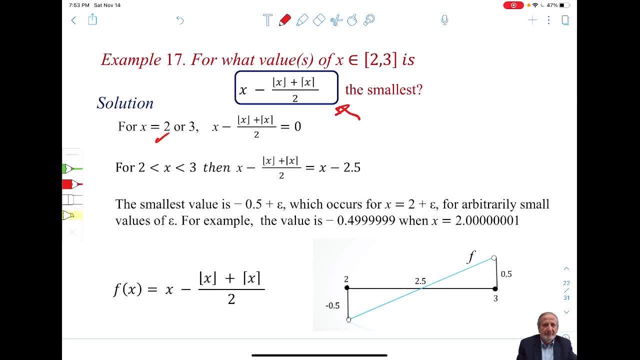 When X is 2, you get here On top. here you get 2 plus 2, 4 divided by 2, 2.. 2 minus 2, you get 0.. When X is 3, 3 plus 3, 6 divided by 2 is 3.. 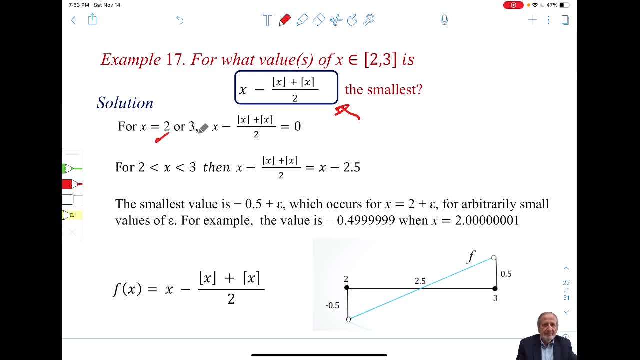 3 minus 3 is 0.. So when X is 2, it's 0.. When X is 3, it's 0. So now I need to have X between 2 and 3.. You make some calculation and you find this is equal to X minus 2.5. 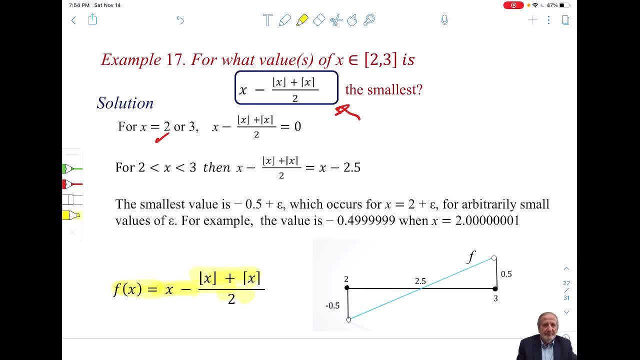 So this function here is equal to X minus 2.5.. So if you draw this function, you find this graph right here. So at 2, it's 0.. At 3, it's 0.. As soon as you move a little bit here, it drops to negative 5.. 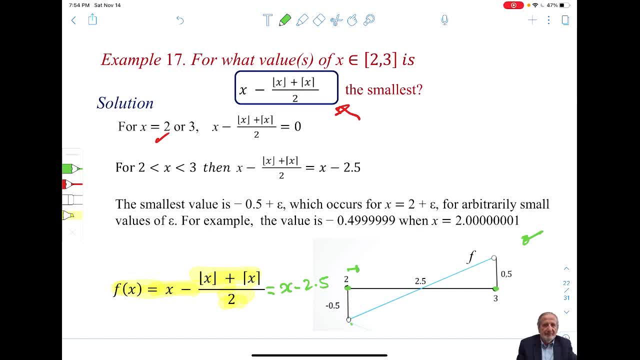 It will not get to the point: negative 5, close to negative 5. And that's the smallest, And then start increasing. So all what you have to do is add an epsilon amount to X to get a very small number. So, for example, the value is minus 4.99999, minus 0.4999 when X is 2.0000001.. 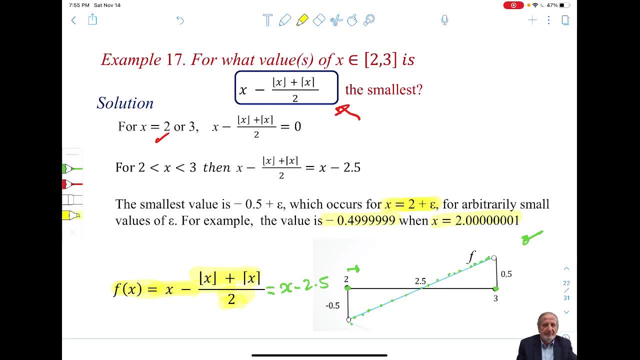 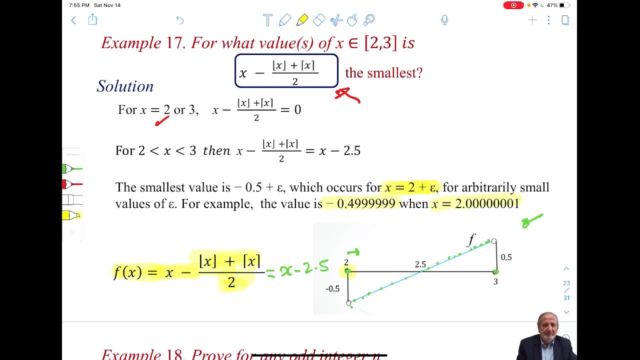 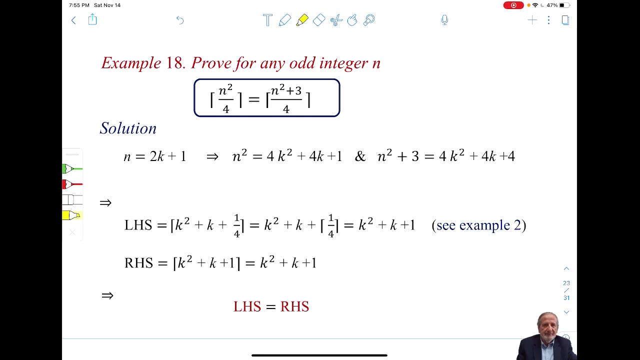 So it will look very close to negative 5, but it will never reach negative 5 because it's 2 when it's 0, when X is 2.. Now we are using solving this. We are using algebraic equations that involve seeding function. 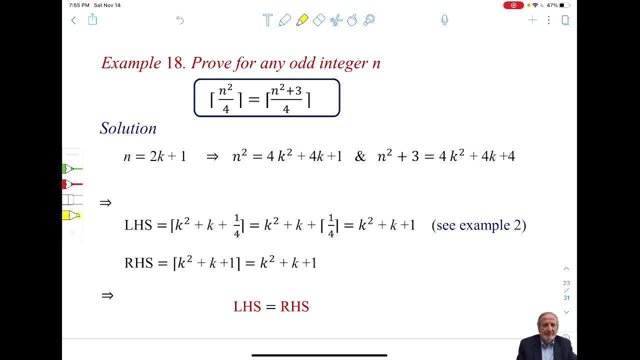 So prove that N square over 4 seeding function is equal to N square plus 3 over 4.. So when N is odd, see N is odd. So now what you have to do is: when N is odd, N means 2K plus 1.. 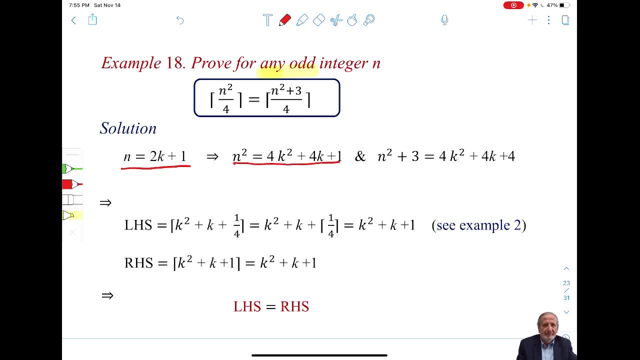 Find N square. Find N square plus 3.. Now, left-hand side, Left-hand side, Find this and divide it by 4.. When you divide this by 4, again, look, what happened is this is an integer. I'm going to get it outside of the bracket. 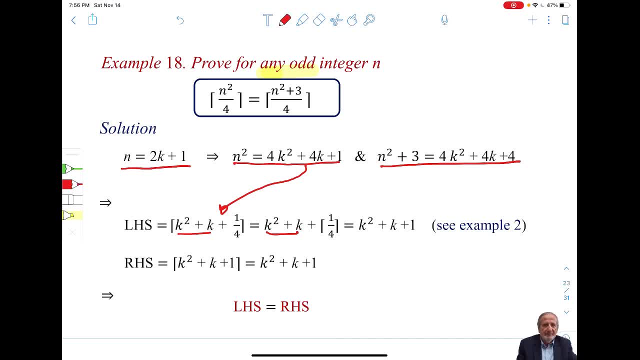 Outer, plus seeding function of 1, fourth, which is 1.. So that's your left-hand side. The right-hand side is: you take this one here and divide it by 4.. And the seeding function, that's an integer itself. 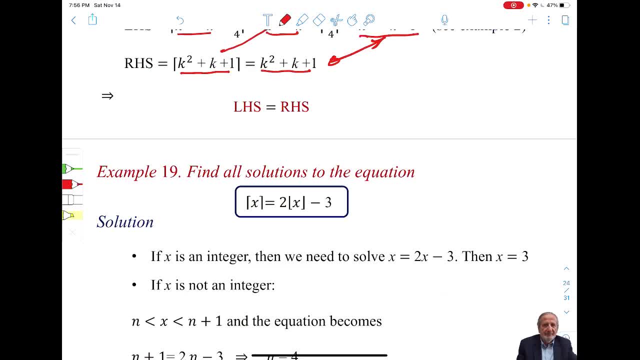 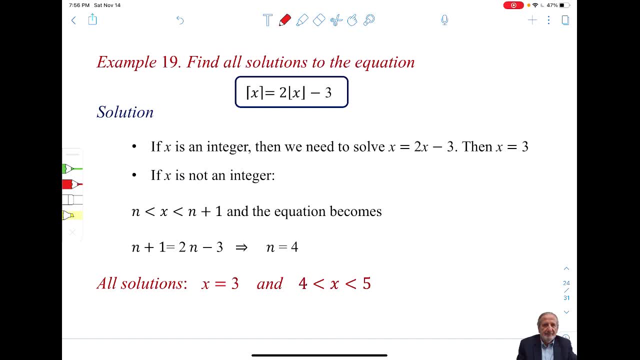 And you see how they are equal. Here is we are solving now solution. What are? find all solutions to the equation. Now, if X is integer, then you have to solve: X is equal to 2X minus 3.. And easily you can find X to be equal to 3.. 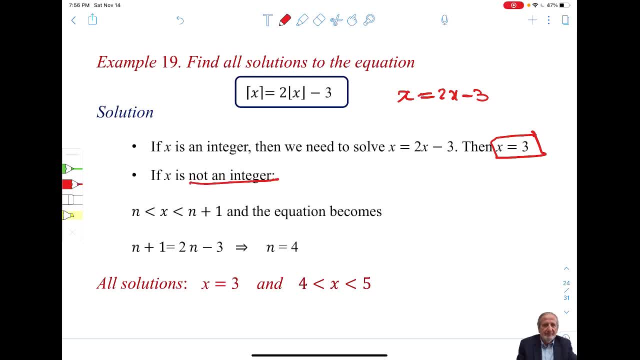 Now X is not an integer, So X is between- we did the same technique- between N and N plus 1.. Let's replace this equation Now. we know: X between N and N plus 1.. So the seeding function of X- the left-hand side here you see- is N plus 1.. 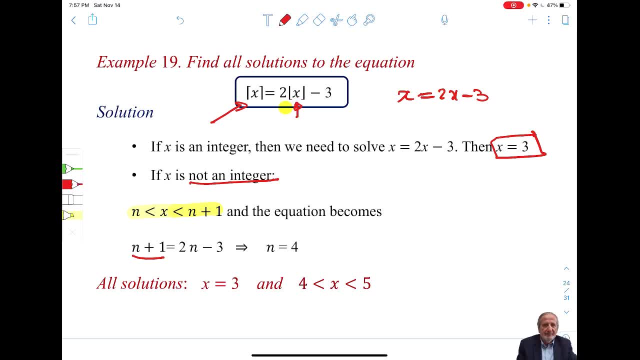 And here you have 2 times the floor function of X, Floor function of X. Floor function of X is N, So 2 times N minus 3.. When you solve this equation you find N is equal to 4.. So now all the solutions are X3 or X, between 4 and 5.. 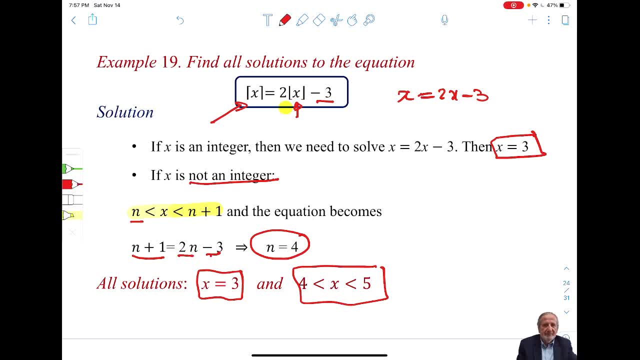 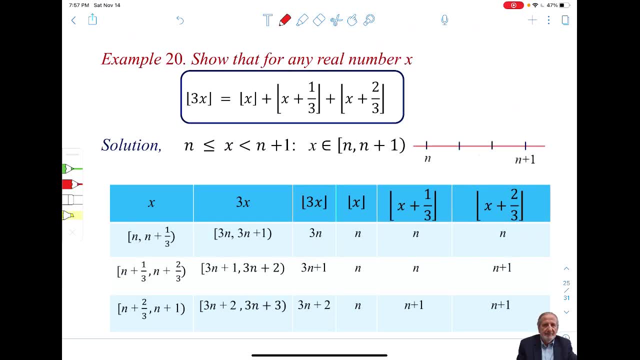 And you can check your answers. Just take 4.2 and see what happens. You find it. you find the left-hand side is equal to the right-hand side. The last example here is: show that for any real number, X, floor function of 3X is floor function of X plus floor function of X plus 1 third, plus floor function of X plus 2 third. 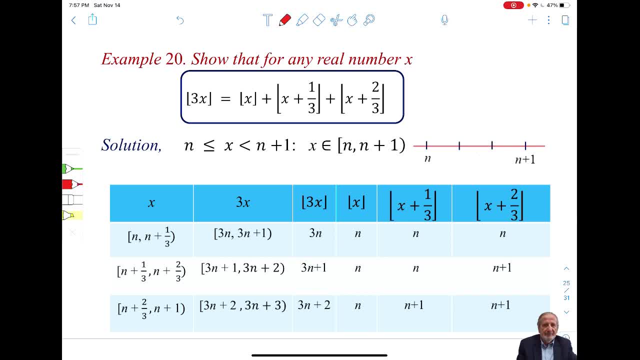 Again, like I did before, I'm going to put X between N and N plus 1.. When I included here X greater, equal than N, I also included in this demonstration the possibility that X is integer, So I don't have to distinguish that case. 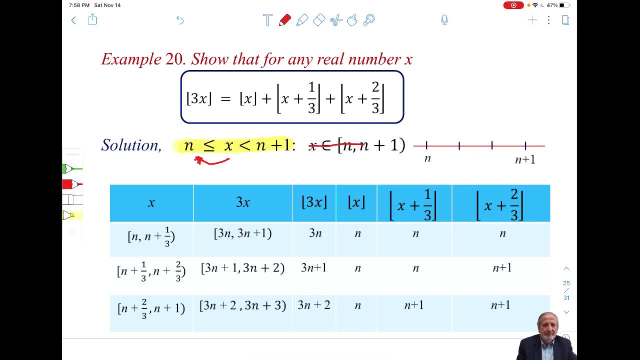 It's already included here. So now this is the same as X in this interval. So now I know X is going to be here between N and N plus 1.. Now the problem here is sometimes I'm adding 1 third. 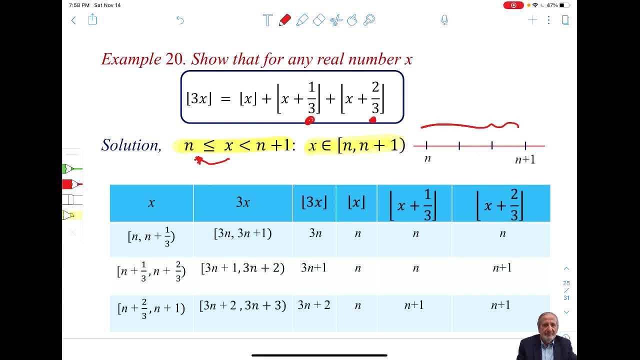 sometimes I'm adding 2 third to the floor function. So it depends: if my X is here and you add 1 third or 2 third, you are still in this interval where the floor function will be N, But but if your X is here, 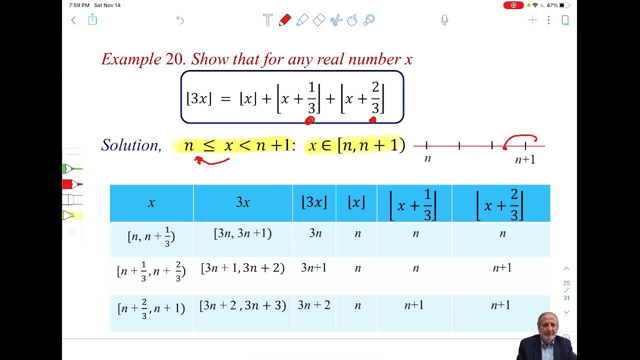 you add 1 third and you add 2 third, you're outside here. then the floor function will be N plus 1.. That's why we are distinguishing three cases: This case, this case and this case. So what happened is X between X in here or here or here? 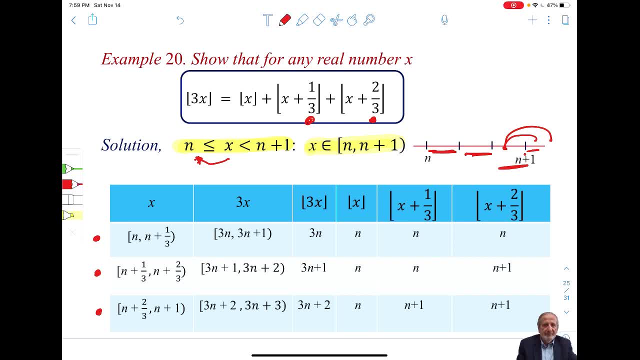 because I have to cover all the values of X, X between N and N plus 1.. So in this case, here you multiply by 3 because I need 3X. You get this Now. what is the floor function of 3X? 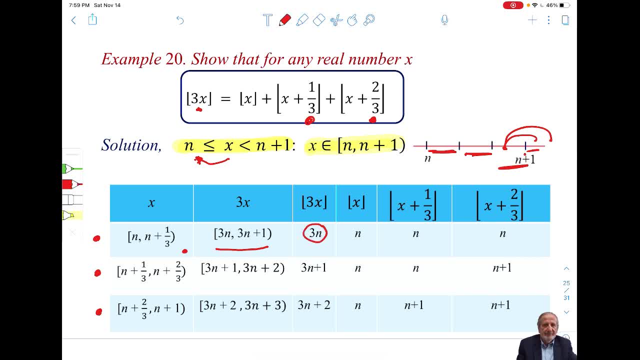 It's 3N. What is the floor function of X? It's N. Now I am here. now. If I add 1 third, or if I add 2 third, I'm going to still be between N and N plus 1.. 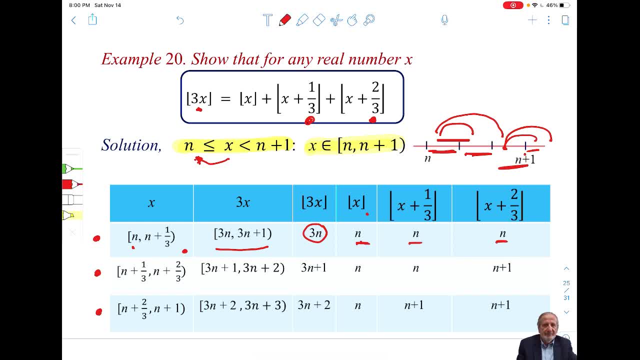 That's why the floor function will be N here, N here and N here. When you add these three together, you get 3N. Now you do the second situation: here: Now your X is your X now is here somewhere here. 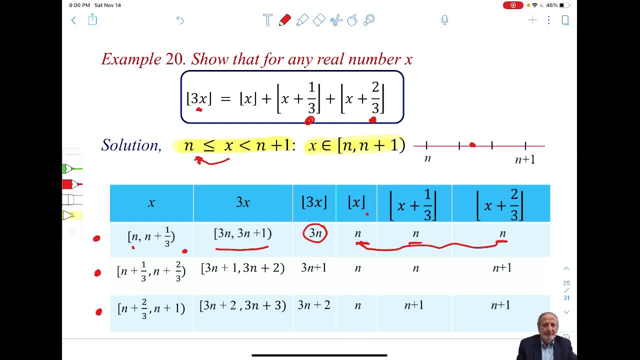 Okay, Now look at here. 3X is this one. So what's the floor function of 3X? It's 3N plus 1.. So I have that. That's the left-hand side. I'm working now on the right-hand side.